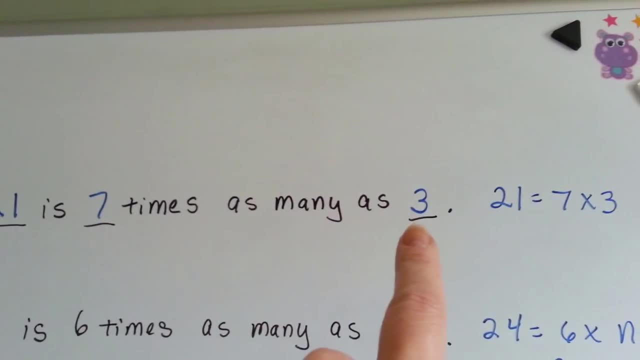 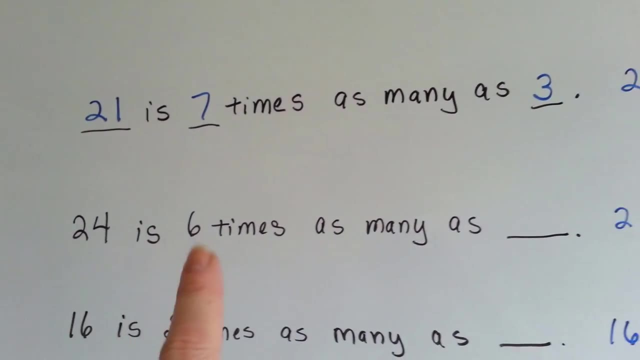 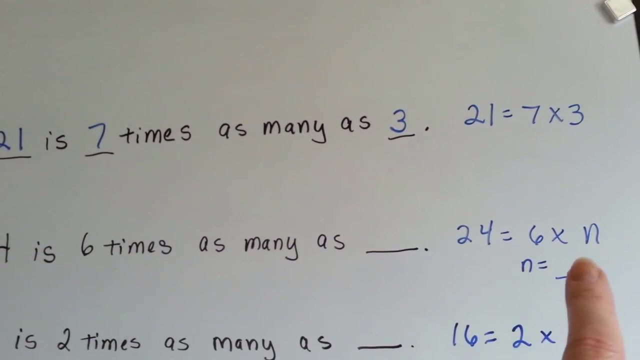 21 is 7 times as many as 3, because 21 is equal to 7 times 3.. Let's try this one: 24 is 6 times as many as 24 is equal to 6 times what. What would n be? 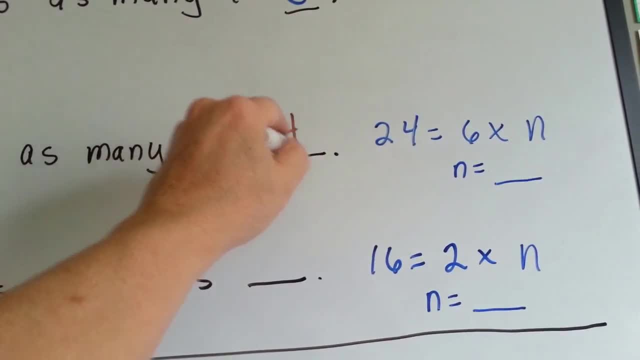 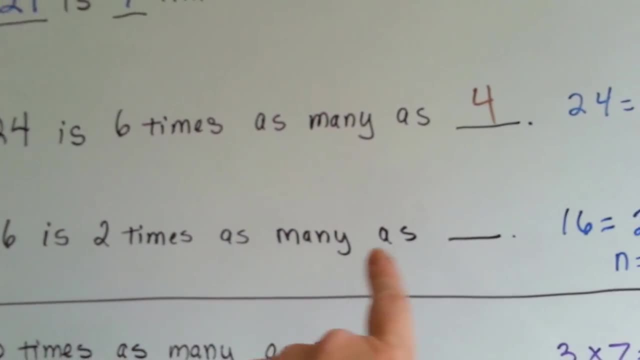 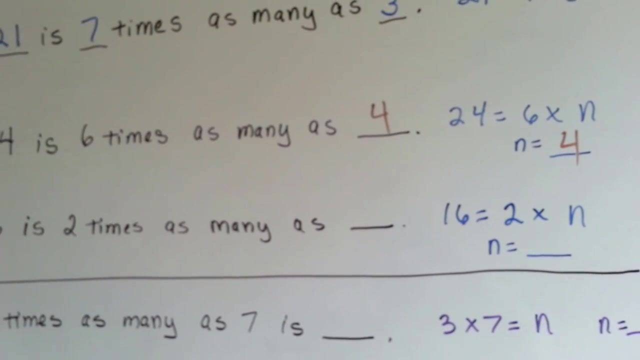 It would be 4.. 6 times 4 is 24.. four, See that Sixteen is two times as many as what. Sixteen is equal to two times n, What is n Two times what is sixteen Two times eight. So do you see how I'm getting? 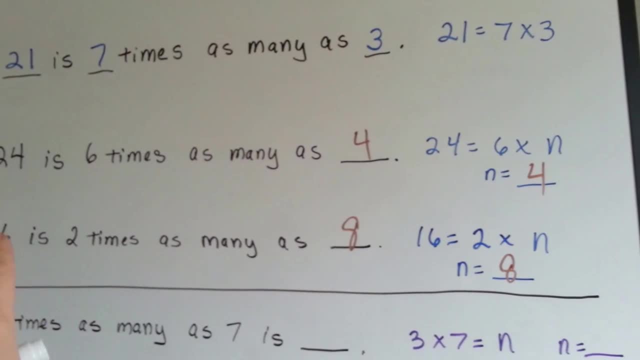 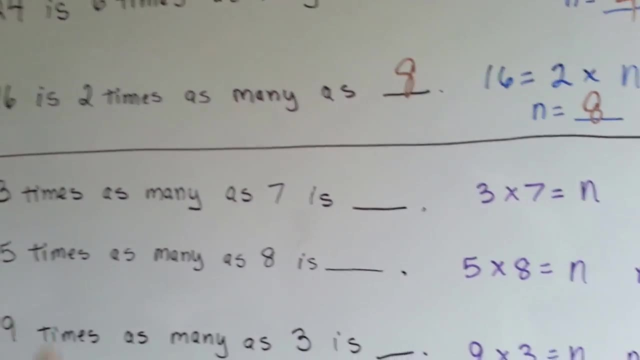 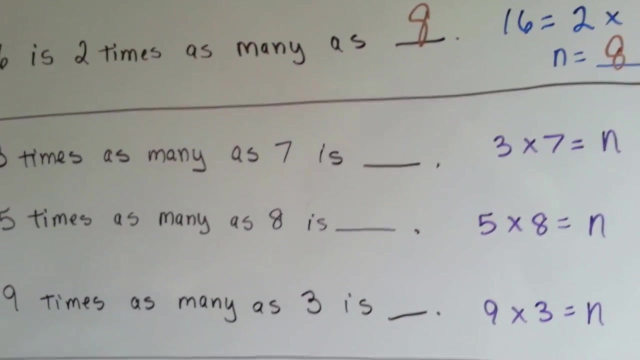 this. It's almost like we're doing the problem backwards. Sixteen is two times as many as eight. See that. Let's try this one. It's worded a little bit different. Now we don't have the big number in the front, It's going to be in the blank space- Three times as many. 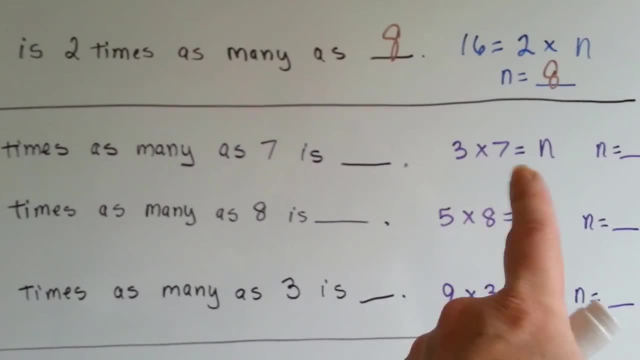 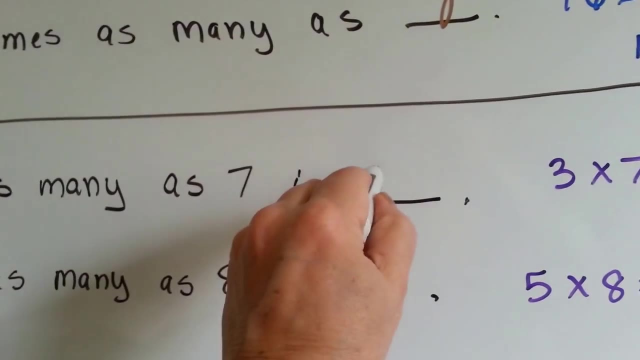 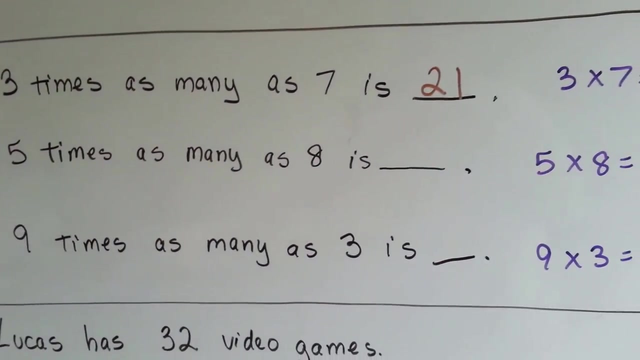 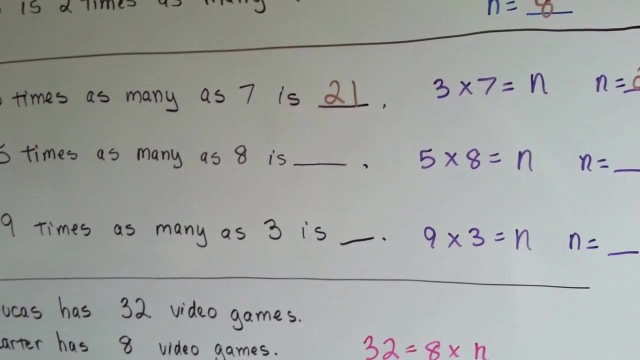 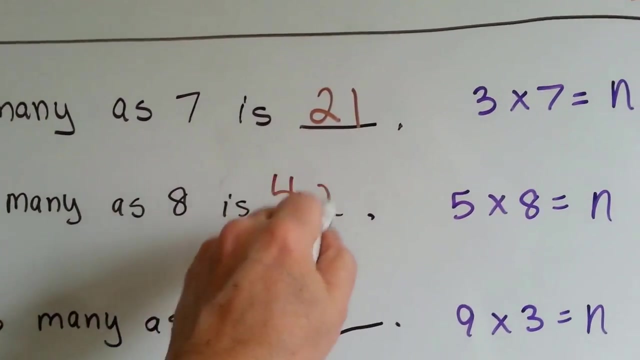 as seven is That's like saying three times seven. Three times as many as seven means three sevens, That's twenty-one. See, Five times as many as eight is another way of saying five times eight. So what is five times eight? Five, ten, fifteen, twenty, twenty-five, thirty, thirty-five, forty, It's forty. So 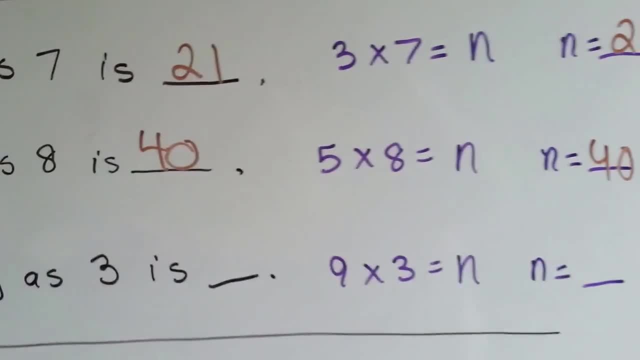 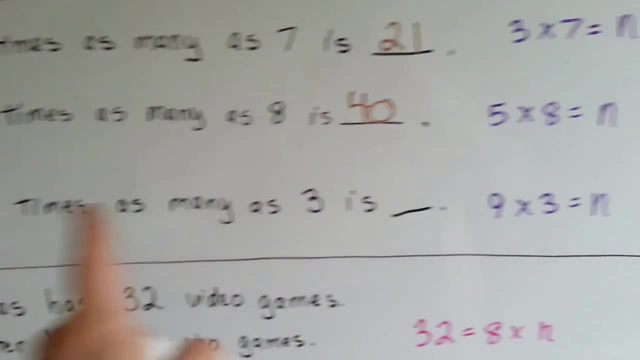 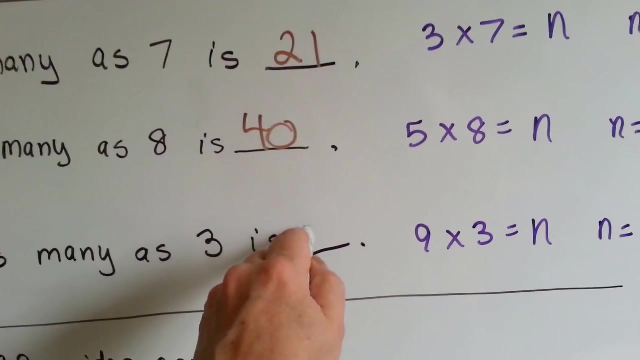 n is equal to forty, Because five times eight is forty. See that Nine times as many as three. So what is nine times three? It's another way of saying nine times three. Nine times three is twenty-seven. N is equal to twenty-seven. See that: 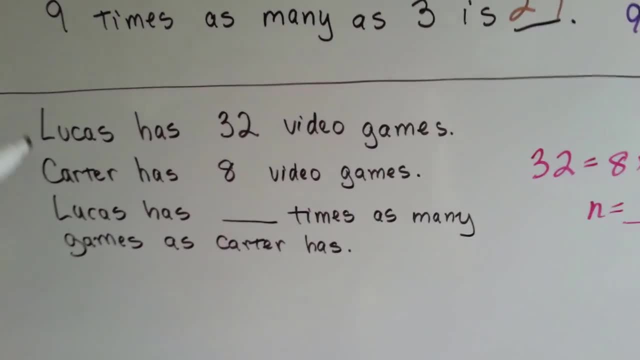 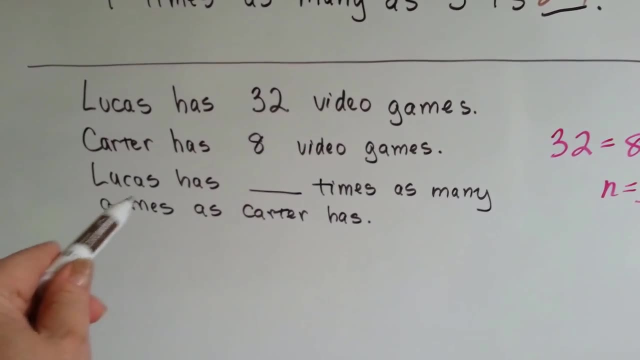 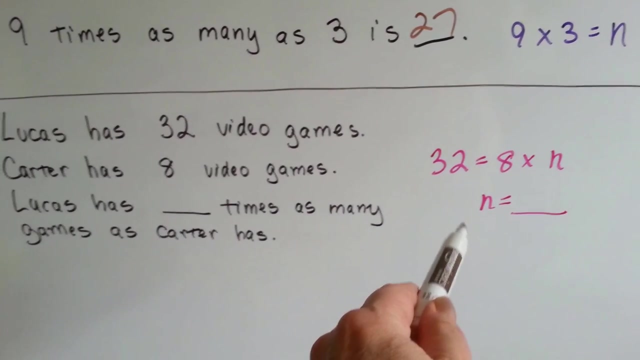 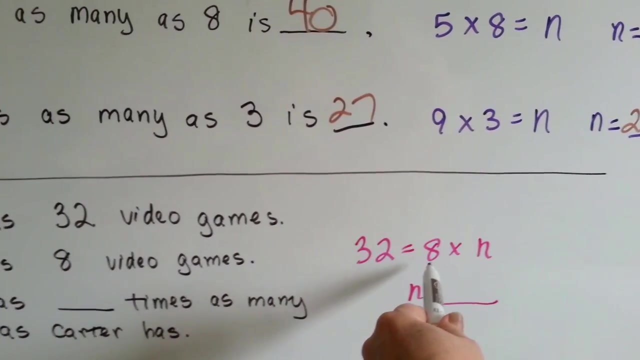 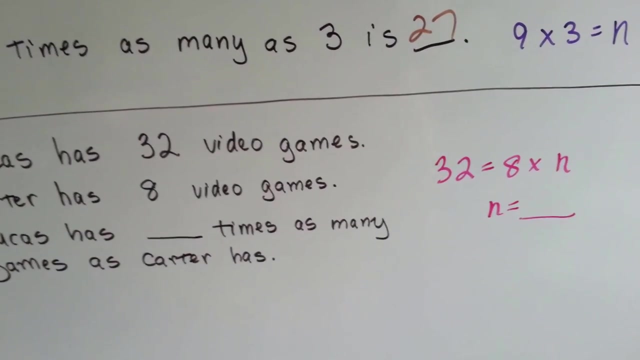 Alright, now let's try this one. Lucas has thirty-two video games. Carter has eight video games. Lucas has blank times as many games as Carter has. So this is how we would write it as an equation: Lucas has thirty-two, Carter has eight. So how many times N times as many games as Carter?